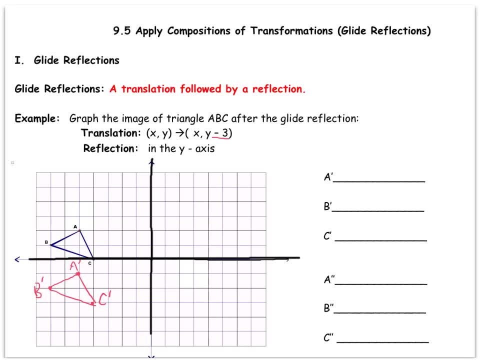 so that would be negative five and down one Negative five, negative one. The others are found just the same. Now the second step is to take the reflection across the y-axis. So we're going to reflect across this vertical, So that's our mirror in this case, and each point needs to be reflected at a right angle. 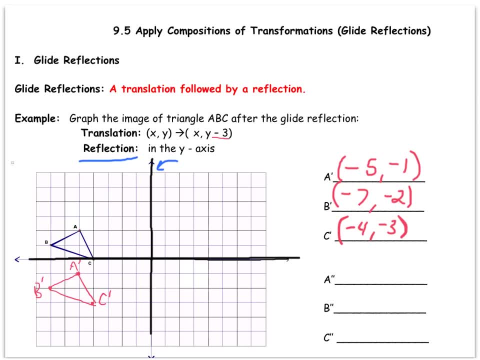 So c prime is four units away from the line of reflection. So we're going to go four units in the opposite direction. Notice, when we're reflecting across the y-axis, what happens to the coordinates is the x value swaps signs. So now this is positive four and negative three. 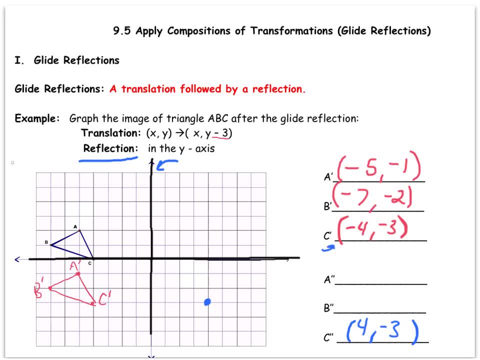 So again the sign. It has just switched in the x component and that's going to be the same for all of them, which leaves us with positive five, negative one and positive seven, negative two. To plot those points, we've got positive five, negative one showing up here. 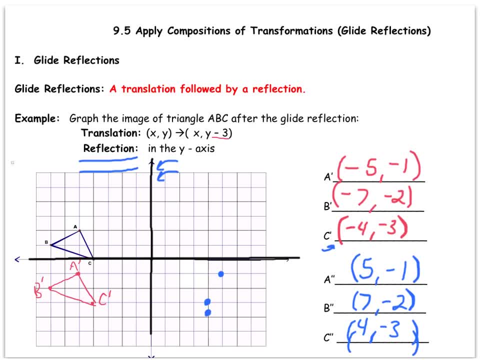 and then for b double prime, positive seven minus two here and we can connect all those points. Make sure you're labeling them. So we have a double prime, the image of a prime, c double prime and b double prime. So this triangle triangle- a, b, c, double prime, all of them, that represents our glide reflection. 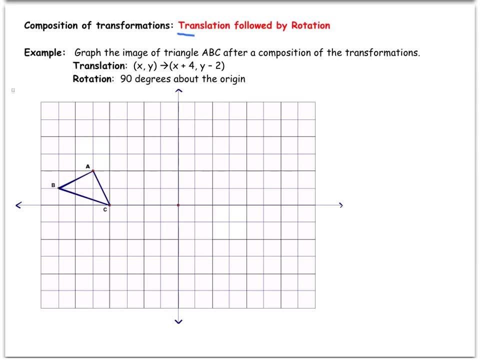 A second example of the composition of transformations is a translation, which we're then going to follow with a rotation. So we'll start with the translation And the translation is: So, each of these values, we're going to move over four, one, two, three, four to the right and down two. 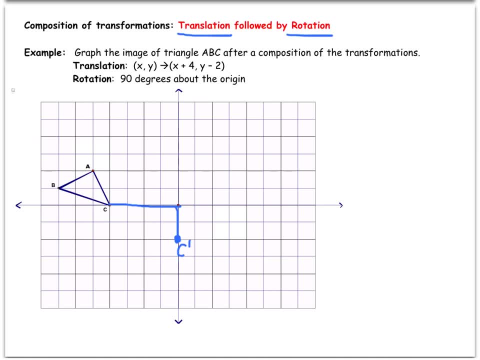 And I'm going to do that for all of them. So here's c prime. A is going to move over four and down, so this is going to be a prime, And then, lastly, b. moving to b prime would be: 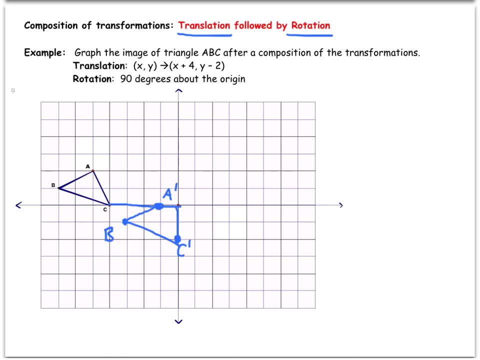 And I can connect that figure. So now this is the image of my original triangle, But now I have to rotate this 90 degrees about the origin. Remember that for a rotation of 90 degrees, what we do is we take a and b. 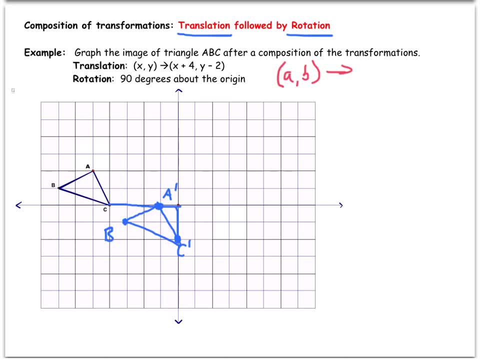 and the translation is reversing a and b but making b now negative. So it's the negative y value Comma the previous x value. I think this is a bit easier if we first list the coordinates of a prime, b prime and c prime. 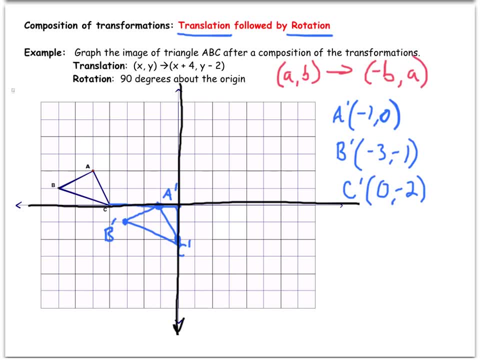 Which gives us negative one, zero for a prime, negative three: negative one which is b prime and c prime is zero, negative two. So now to find a double prime, the rotation of my prime image, I have to switch the x and y values. 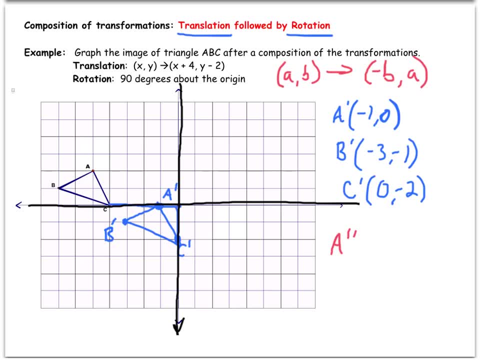 So now to find a double prime, the rotation of my prime image, I have to switch the x and y values and change the sign of the new x. So I'm going to first switch them: negative one and zero swap around. 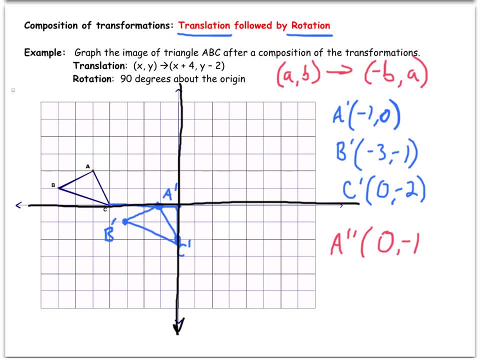 and I make the zero negative, but zero, negative, zero. they're the same thing. So my new coordinate is: a double prime is zero negative, one b prime. first start by swapping the two negative, one, negative, three, and then changing the sign of my new x value so it's going to become positive one. 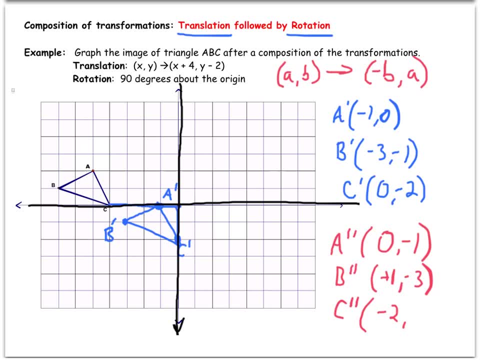 And then c double prime: swap the two negative, 2 and 0, but the x value now becomes positive. Last step: I have to graph all of these: 0, negative 1 will be my a double prime: positive 1,, negative, 3,. 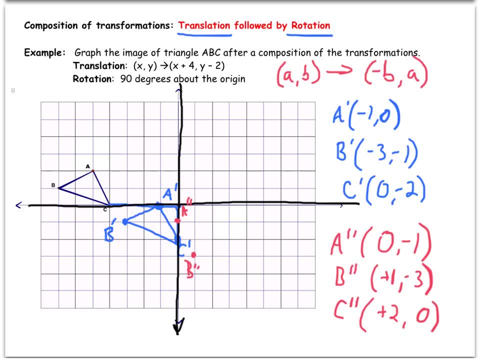 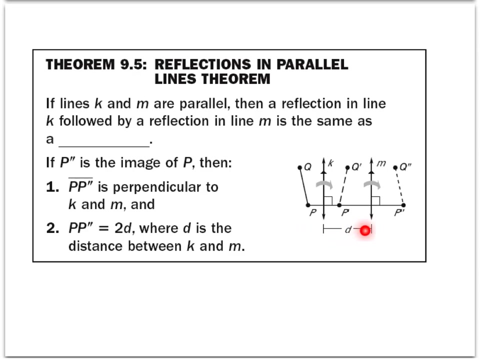 b- double prime and c- double prime at 2, 0.. And now I've shown the composition of the transformation, coming up with my image being the final prime image in the red. You may have stood in front of a few mirrors before and 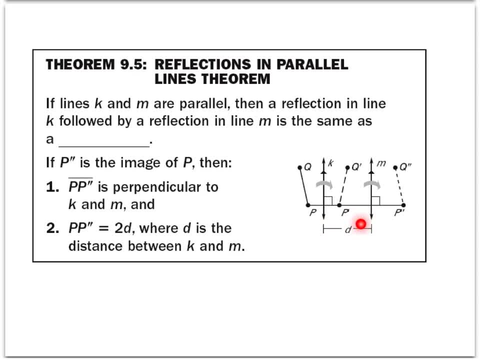 been wearing a shirt that had letters on it and realized that in one of the mirrors, your shirt read all of the letters in reverse or flipped upside down. and then the other one. the words were able to be read again, And this is a property that we can study. so what we need to have, 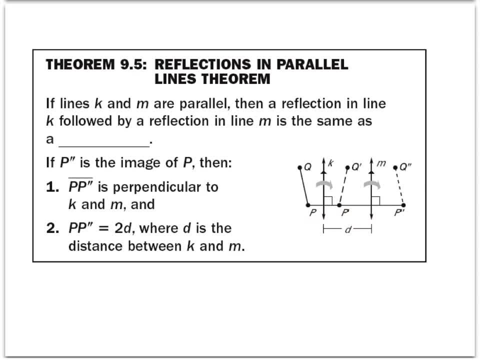 happen is we have two mirrors, for example, or, in this case, two lines of reflection- k and m- that are both parallel to one another, And what happens is you start with the original image, so the pre-image, and that pre-image is reflected across the first. 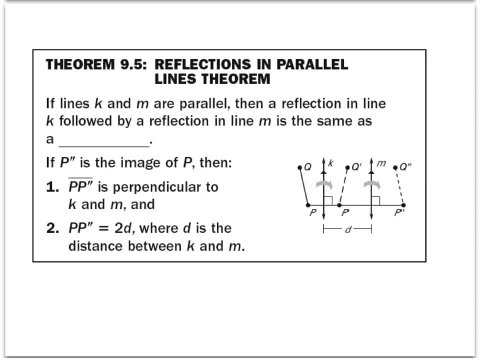 line giving you q prime and p prime, which is then reflected again, and this brings you back to the original image. It's the same orientation. however, now it's been shifted over, So it's been translated. So, if k and m are parallel, then the reflection in line k, followed by a reflection in line. 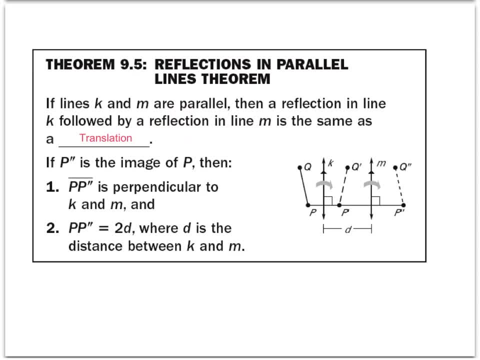 m is the same as a translation. This brings up two important points. So we're going to look at p prime and this is the image of p, And what happens is the line segment formed between p and p prime has to be perpendicular to both lines k and lines m, and we've looked at that. 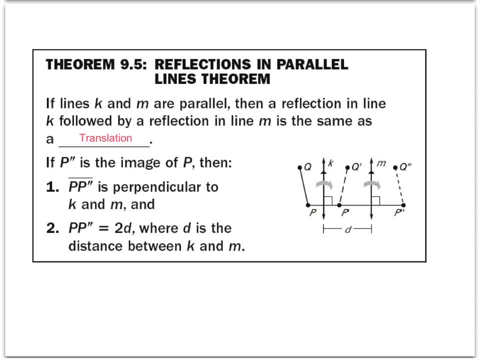 before in terms of reflections and how they land at a perpendicular point. So this means that this is going to differentiate from one line to the other. So the reflection in line k and the reflection in line p is going to oston at a perpendicular point. 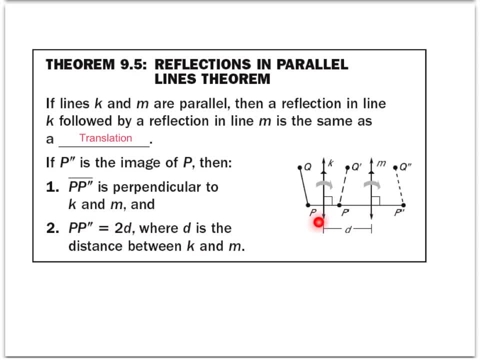 So, for example, k prime is going to be the distance between the lines p and m, and p prime is going to be the distance between lines k and line m, And the expression for the line segment is going to be the distance from the angle of the angle to each of the mirrors. 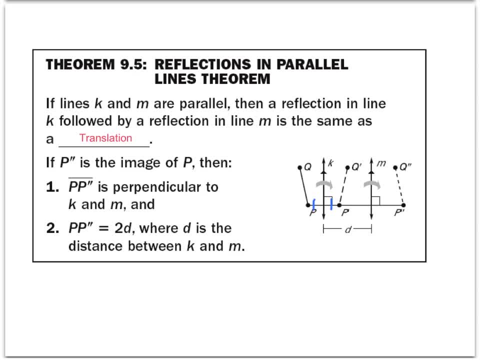 Second, p, prime is going to be a section formed from P to the image, So it has to be two times or twice the distance between these two parallel lines, prime to m, based on the properties of reflections. So what we can do is add them together. We have 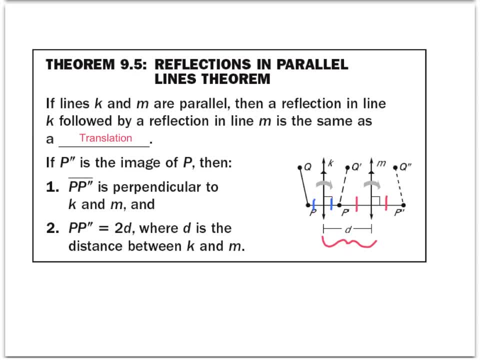 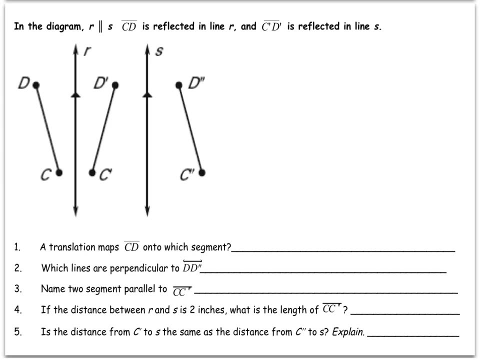 the distance here is represented by the blue segment and the red segment and the distance on the outside is also a blue segment and a red segment. so that's twice the distance Using these properties. we have again two parallel lines given here and we have line segment CD is reflected. 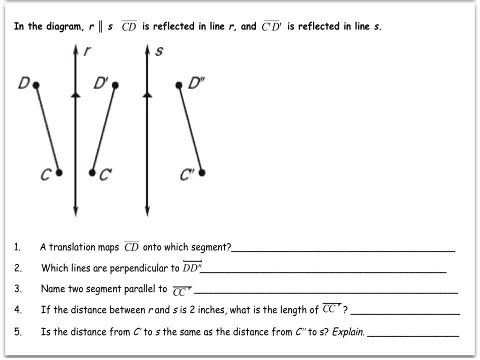 about the line R giving us C prime, D prime, which is then reflected about the line S. First question is: a translation maps segment CD onto which segment? Well, this translation is going to move C over to C prime and D over to D prime, so this is going to be segment C: double, prime D double. 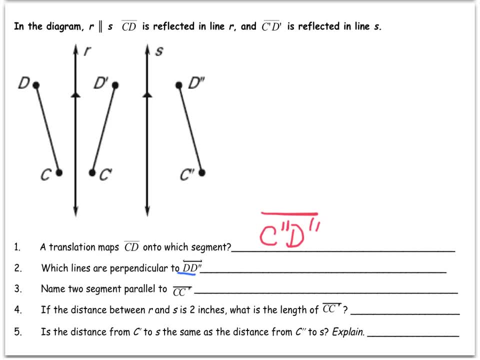 prime perpendicular to line D, D prime. Well, let's form that line first. so we have this line here which should be perpendicular to each of the lines by the properties of reflection. So which lines are perpendicular? Both lines are perpendicular, line R and line S. Looking at, 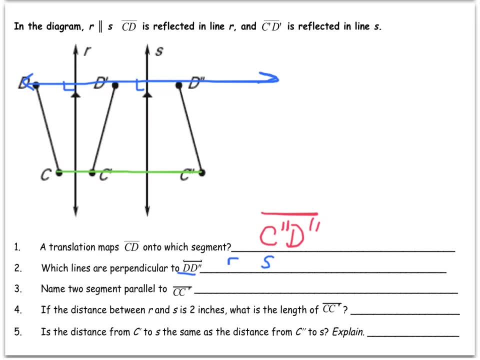 segment C- C prime. we're asked to name two segments that are parallel to C- C prime. so clearly, one of the segments could be D- D prime and then a second one could be D prime- D- double prime. so we'll write C prime, which is parallel, and D prime, D double prime. Now we know that these are parallel because we 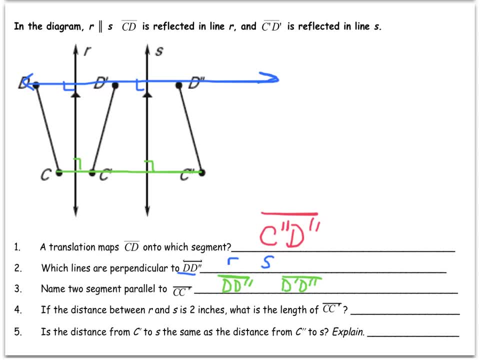 have that this segment is perpendicular to both the lines. so we have two lines that are both perpendicular, same lines, making them parallel, Given that the distance between R and S is two inches, meaning the distance between these two lines is two inches, when asked what the length from. 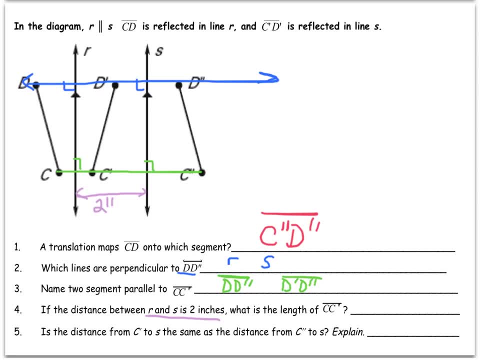 C to C double prime is all we have to do is take and double that, because this total length is going to be twice the distance between the two lines. so two times two, which is four inches. Lastly, we want to know: is the distance from C prime to C double prime equal? are those congruent and, as you've 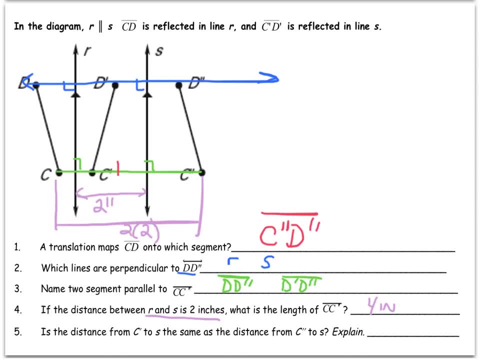 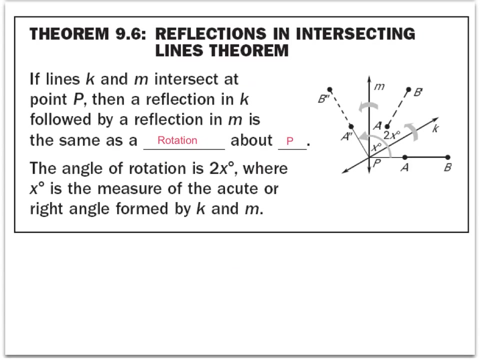 already studied by properties of reflection. these must be congruent. The reflection from C prime to the line and the line to C double prime are the same exact lengths. so yes, they are the same distance. Don't pay too much attention to the name of this theorem, but rather how to use it. 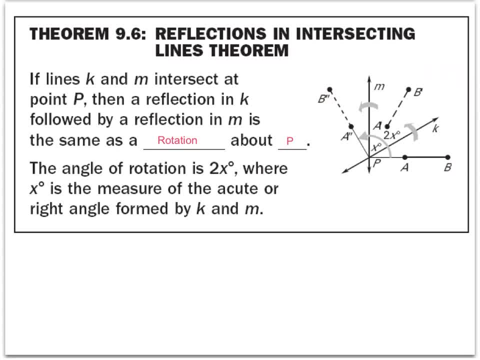 This picture is a pretty good representation of the theorem, but I'm gonna draw it out as we construct it. So what we're gonna do is we're gonna take two lines. we're gonna take the line K and two lines at the top of thekt. 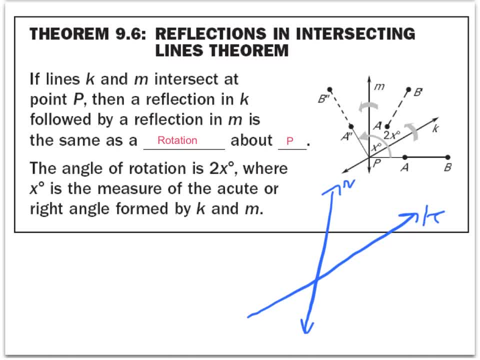 the line M, And these two lines are going to intersect at one point. This point I'm going to label as P, A reflection in K. So if we start with some point, let's just put it right here and we reflect it. about the line. 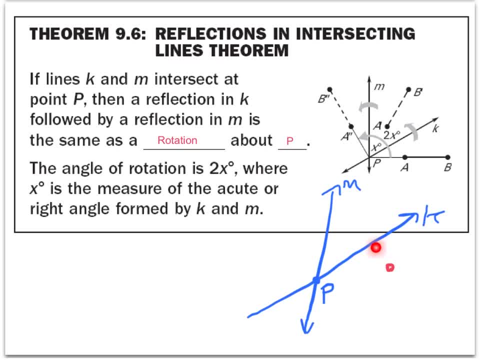 K. So what we're going to do is take this point and drop it perpendicular and put it the same distance over here, The reflection about the line K, So it would end up somewhere about there, And let me label this point. I'll label it. 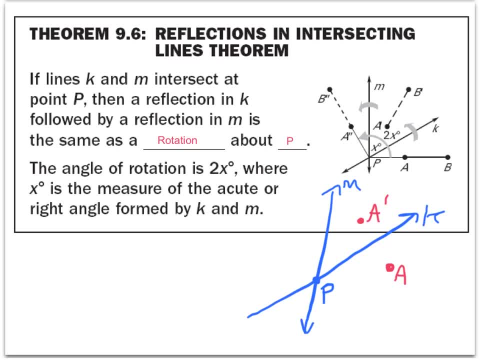 A, So it's reflection is A prime, the image of A, And then I'm going to reflect that one more time about the line M, So right across here, And I'm going to label that A double prime. And what this theorem says is: if you reflect, 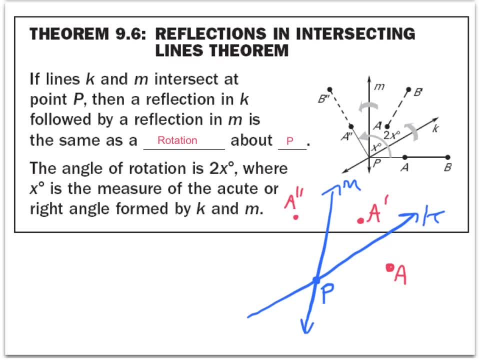 across two intersecting lines. it's the same thing as a rotation about the point P. So where P is the center of rotation, point A is now being rotated about some degree measure around to A double prime And we can actually figure out what the 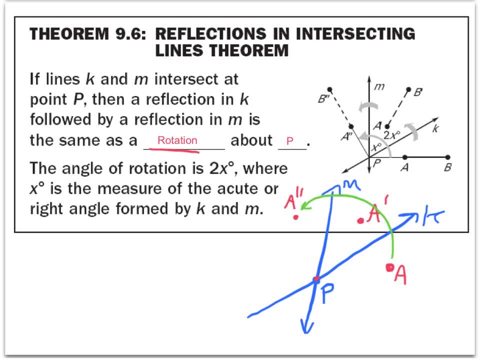 rotation is. What we can do is we take the angle between the two intersecting lines, And what we want to do is take this angle. We'll call it X degrees. We do not want to look at the larger angle, We want to look at the acute or 90 degrees. 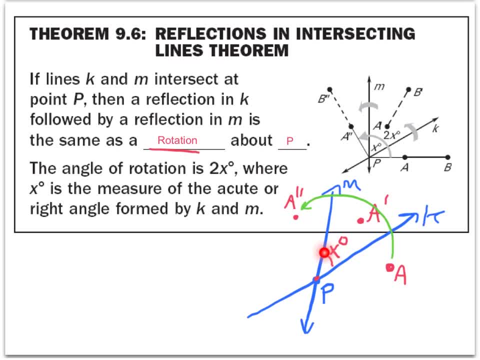 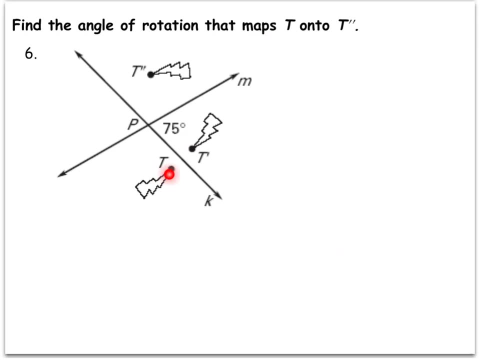 So do not look at this larger angle, but rather the angle in between like this: And the rotation is actually twice this value, So 2 times X degrees is going to be the angle of rotation. Putting the last theorem to work, we've got T. 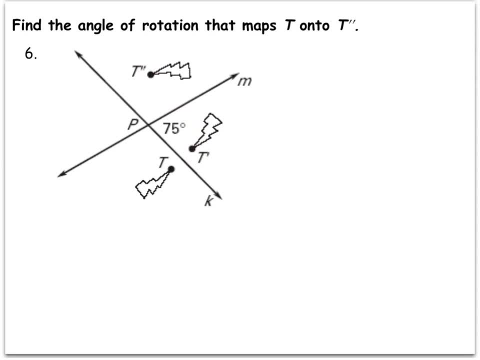 which is then reflected across the line K and then reflected across the line M. So this is going to represent a rotation, since it's reflected about two lines that are intersecting at point P. So now point P becomes the center of rotation, And what we have is we're going to focus on the point here. 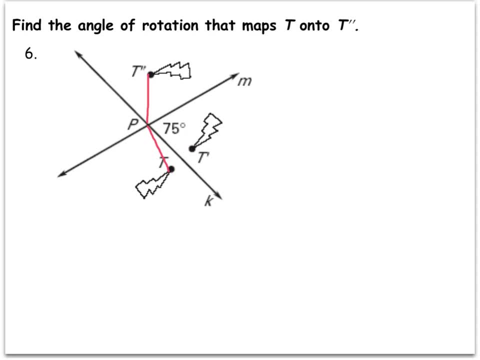 this point, T rotating all the way around to T double prime. So it does one of these, And to find the angle of rotation, what we have to do is look at the acute angle, between which is 75 degrees, and multiply it by 2.. 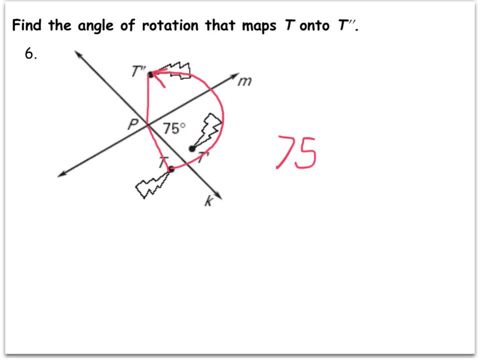 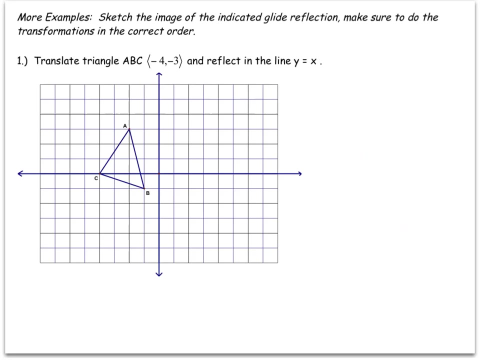 So here we just take 75 degrees times 2. And that turns that by 2, which equals 150 degrees. So this is a rotation of 150 degrees. One last example that we'll walk through is a glide reflection. So we're first going to translate this triangle and then reflect it about the line. 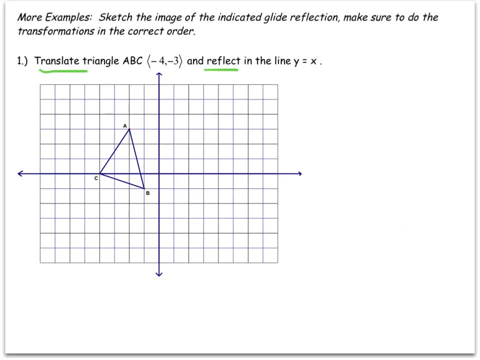 Y equals X. Step 1, the translation. Here we're giving a vector that represents the translation. So we have to take each point and move it to the left 4, since it's negative, 4 in the X direction, And down 3, by negative 3.. So we'll take C. 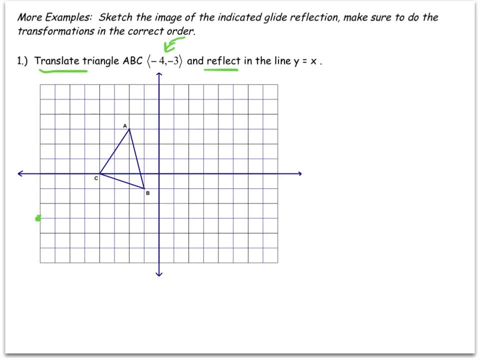 over to the left, 4, down, 3.. Gives us C prime right here. A prime is going to be same thing over, 4, down, 3. A prime And then B prime right here. Connect up those points for my. 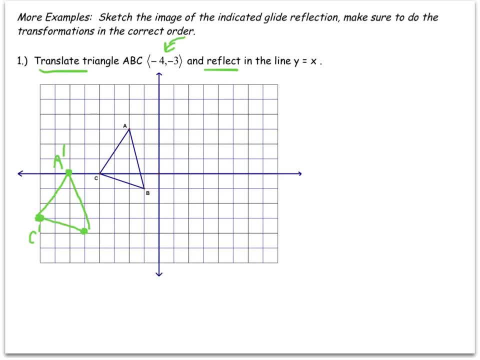 image of the original triangle, Digging up our formulas that we used earlier to reflect about the line Y equals X. we can take the point AB and swap its components, So this becomes B comma A. So each of these points, we can find the coordinate point and just swap them around. 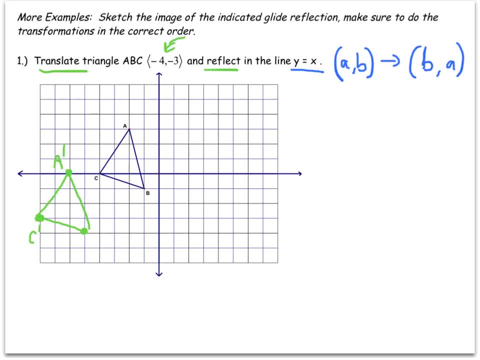 and then plot it And keep in mind graphically what it means to reflect across: Y equals X. That's this line here, The line of slope positive 1 that goes straight through the origin. I find it helpful to first find our A prime. 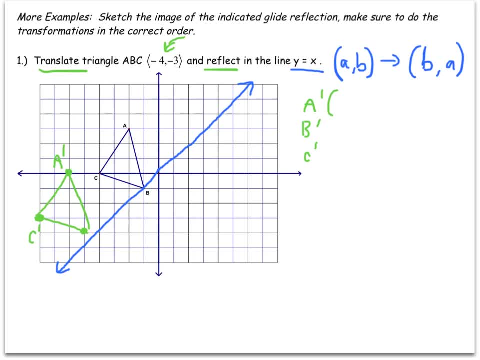 B prime and C prime coordinates, A prime being negative 6, 0.. B prime negative 5, negative 4.. And C prime negative 8, negative 3.. By listing it that way now it's a lot easier to actually plot the others, because I'm just reversing. 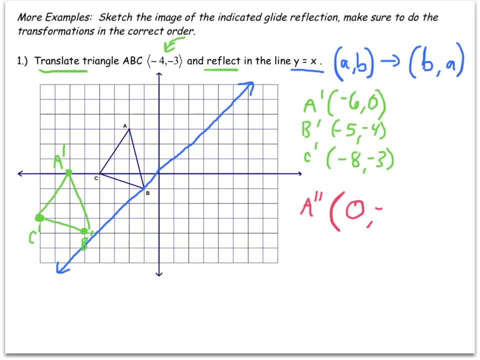 the points: A- double prime: swap the two: 0, negative, 6.. B- double prime: swap the two negative, 4, negative, 5.. And finally, C, double prime, again swapping negative 3, negative 8..